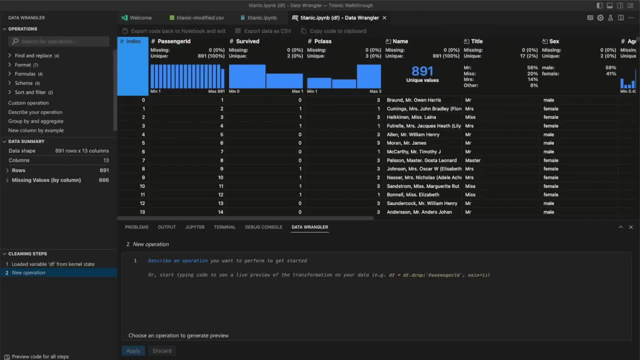 you'll have a completely isolated, sandboxed environment to explore and try out various data cleaning operations without any fear of overwriting the original dataset. So let's start off with taking a look around Data Wrangler. There are six main components. I want to walk everyone through. The first element is the Data Wrangler grid. 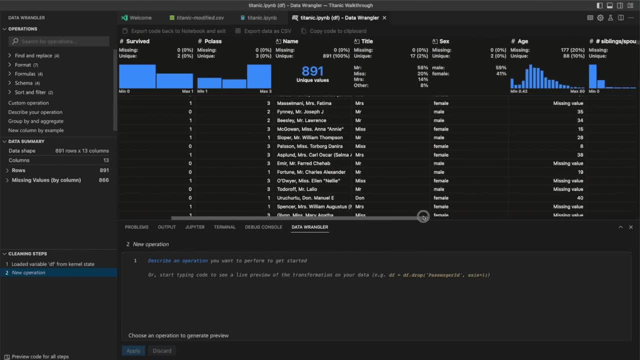 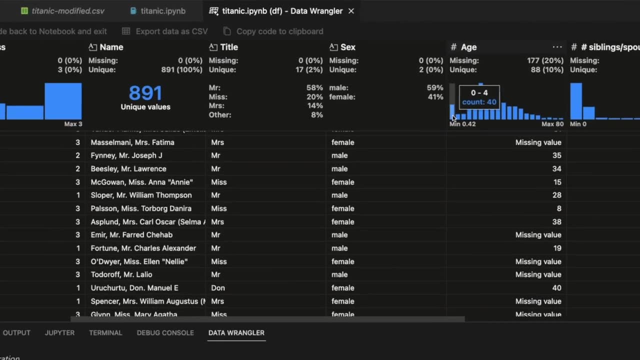 Here is where you can see the full values in your dataset. Later, when we start to clean your data, the grid will also show you a diff of the changes to your actual dataset. At the headers of the grid is what we call our quick insights. Its role is to give you the most. 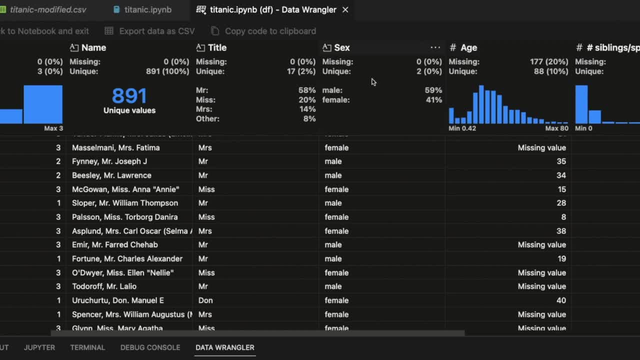 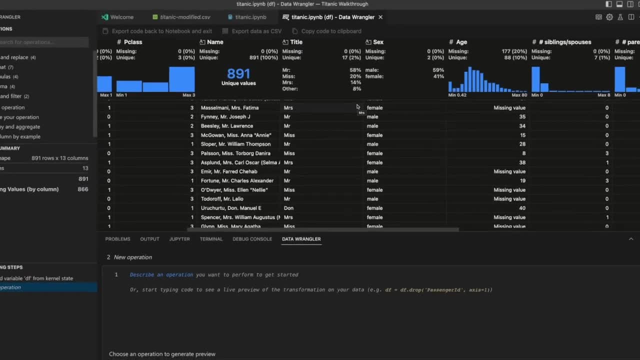 important information about your columns at a glance, Things like the column data type, the percentage of unique and missing values, data distributions, frequency tables, etc. Again, this is automatically all generated by Data Wrangler. On the left hand side is where you'll find the operations panel. 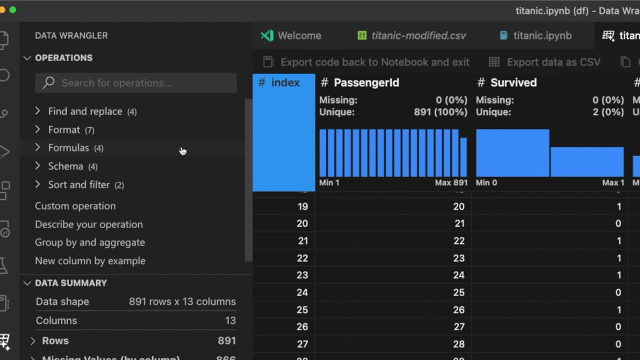 Data Wrangler has many common data cleaning operations built in, and this lets you perform data cleaning and data analysis with ease, as you'll no longer need to look at Panda's APIs or documentation and will be able to see the direct effects of the operation on your data. 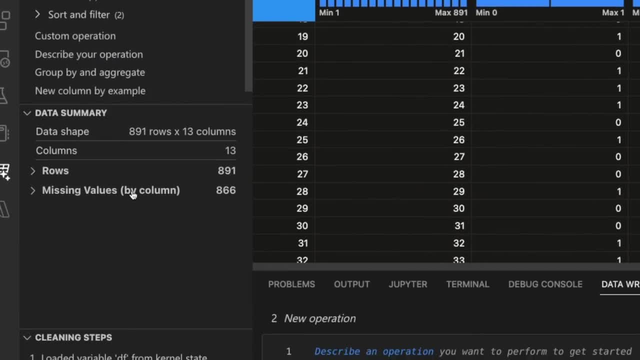 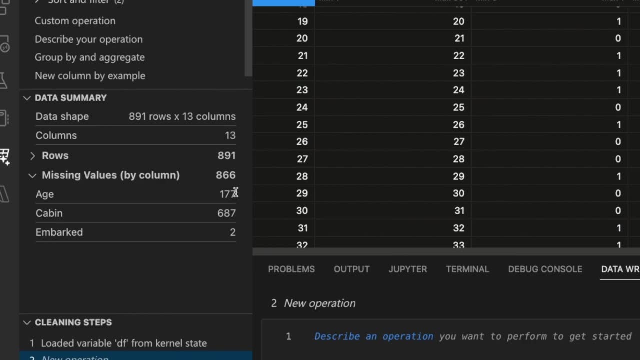 in real time. within the grid Below the operation panel, we have this data summary statistics. When no columns are selected, it shows important information about the entire dataset, such as the data shape and which columns have missing rows. When a column is selected, it gives you more. 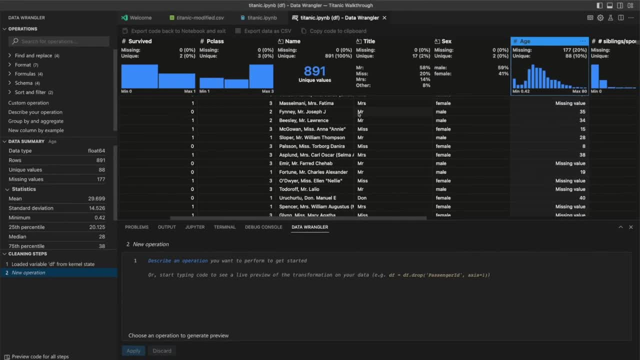 detailed insights about the column itself. If we were curious about the ages of the passenger on the Titanic, we can actually see additional information such as the mean age and other stats such as the skew of the column. We recommend dragging the summary panel to the right. 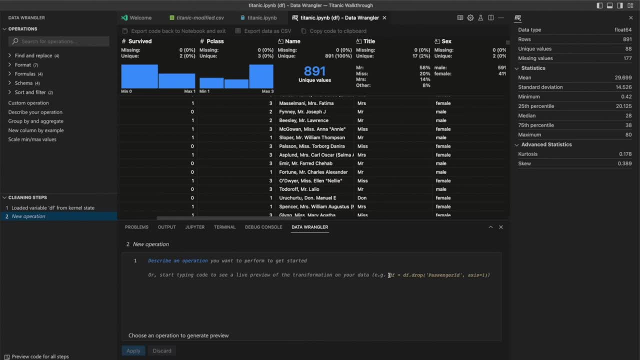 side of the screen for more screen real estate. At the very bottom of the screen we'll have the code preview panel. Here's where you can actually either write Panda's code and see its effects in the grid, or see the automatically generated code from Data Wrangler. 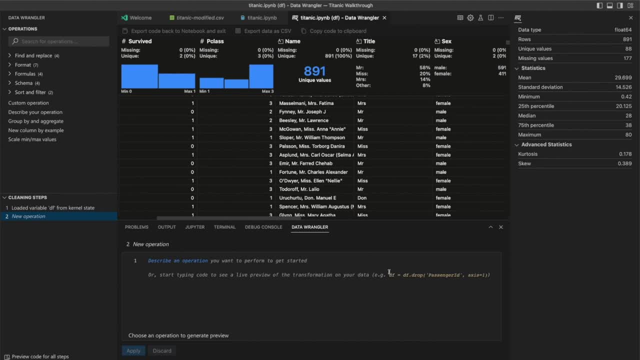 when you perform the built-in data cleaning operations. This will become self-explanatory once we start doing some exploratory data analysis. This will allow us to see the data cleanings that we've done in the past. This will allow us to see the data cleanings that we've done in the past. 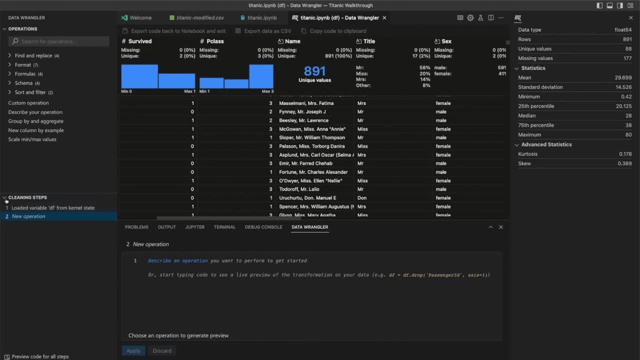 Finally, we have the cleaning sips panel, which holds a log of all the operations you've done to your dataset. When you first launch Data Wrangler it's blank, but you'll start to see it pop up with items as we clean the Titanic dataset Now that we've gotten familiar with the Data Wrangler. 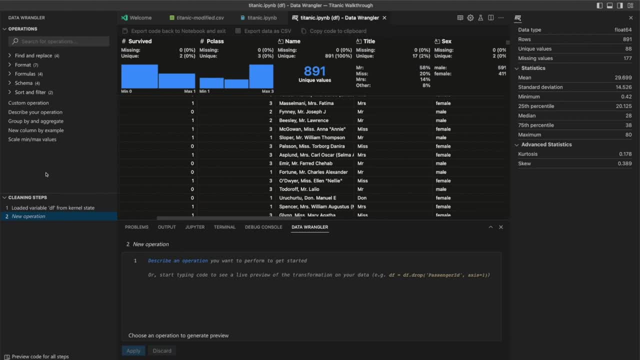 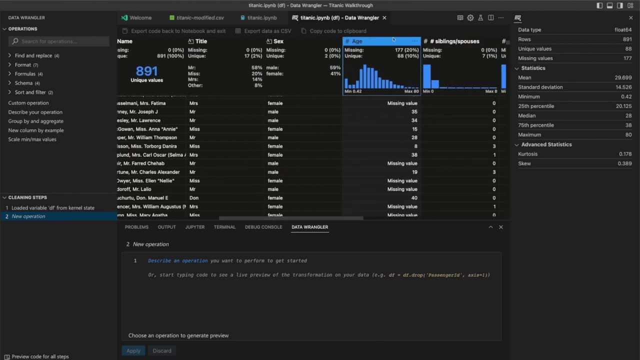 interface. let's use it to clean up the Titanic dataset, to make some better predictions on the survivability of passengers. Firstly, we'll want to know which columns have missing values. since these may be problematic for our future ML model, I'll unselect the age column so that 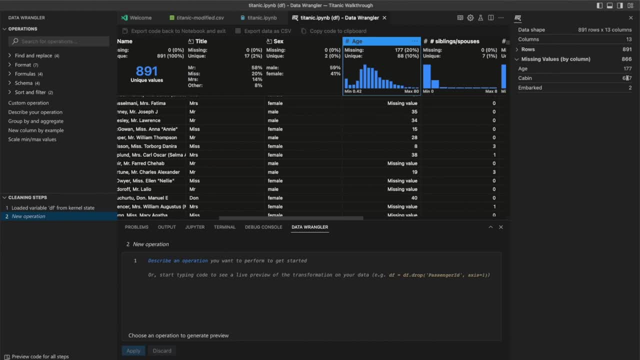 we can see the summary stats for the entire dataset again. We can see that age, cabin and embarked columns have missing values. in this dataset, Specifically, the cabin column has the majority of missing values, so we can just do a simple drop on it. To do so, I can either directly: 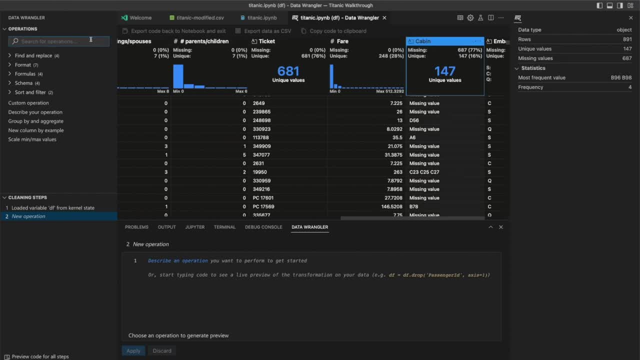 write the pandas code to do it, or I can actually leverage the many built-in data cleaning operations within Data Wrangler To do so. I can just search for the keyword drop in the operation panel and you'll notice immediately that any time you preview a data cleaning operation in Data Wrangler. 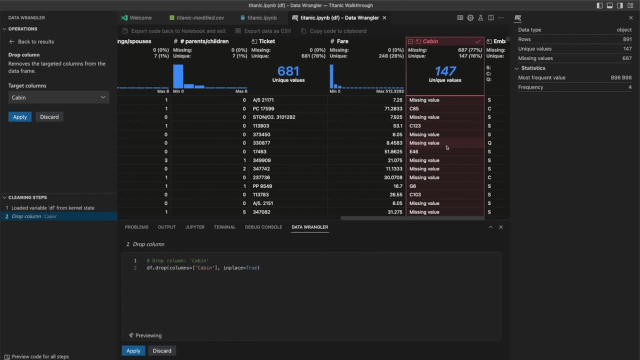 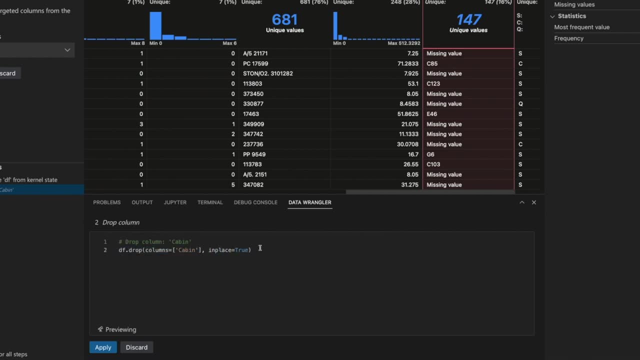 the data grid will showcase what the change in the data cleaning operations will look like. The changes will be to the dataset visually, so you can make an informed decision of whether the operation is what you expected. In addition to the visual preview, Data Wrangler will also generate. 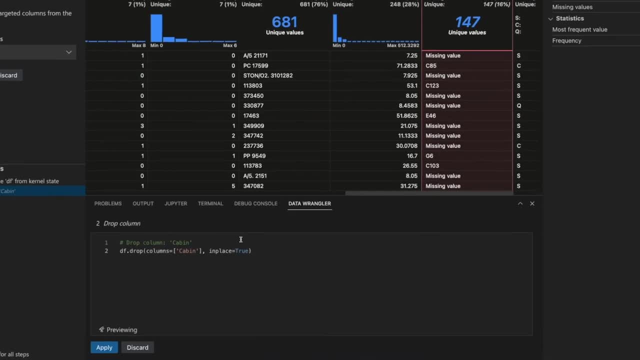 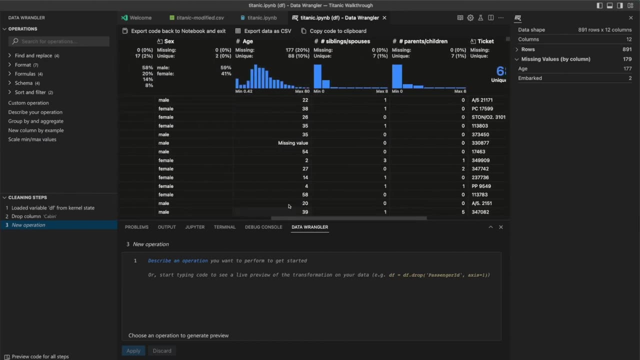 clean and concise Python code for said operation, giving you another means to review and ensure that the operation is doing what you expect it to do. Once it looks good, you can click accept, Moving on to addressing the age column. now, one easy thing we could do is to just remove all the 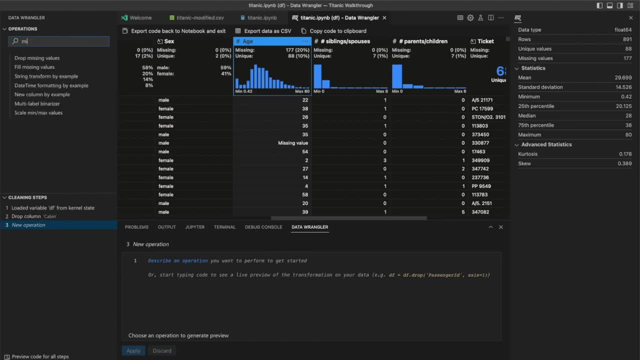 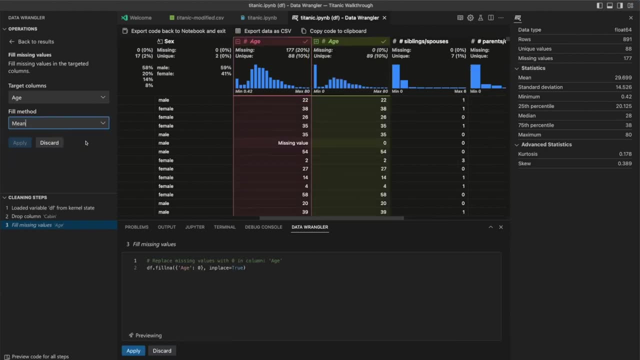 missing values, but since this dataset has so little rows to begin with, we'll want to keep as much of the data as possible. We can start off by replacing the missing values with the average age. Again, you can see the data preview coming in handy, as we now can see how the individual 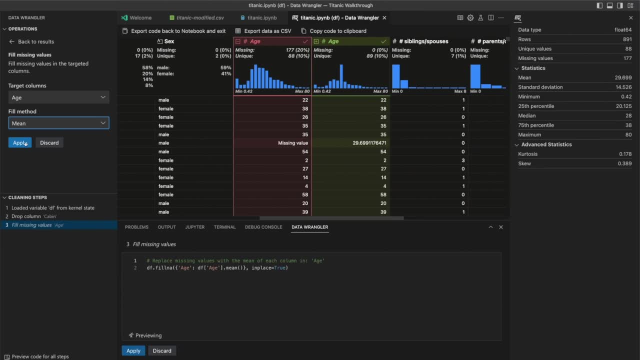 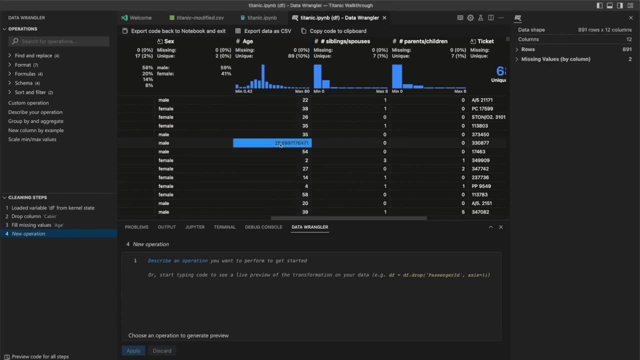 highlighted rows of data change, as well as the change in the quick insights, such as the unique and missing values. After clicking apply, I actually noticed that the mean age is not really a nice integer, so we can actually go ahead and edit the code previously generated by Data Wrangler. 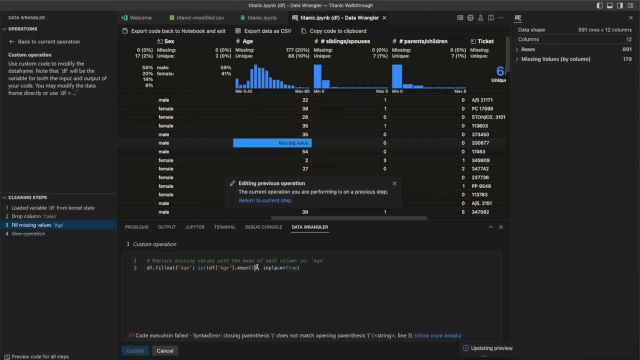 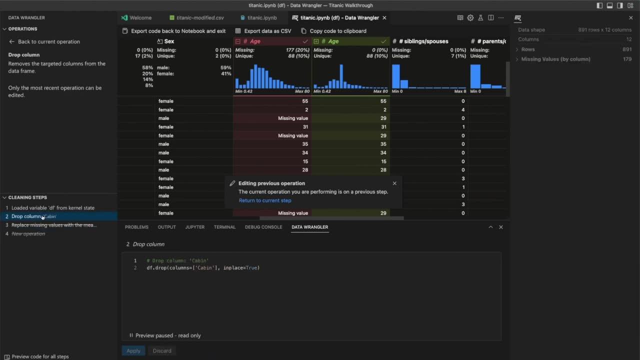 to modify the operation. In this case, we'll want to cast the mean function to be an integer, but we'll also want to make sure that it's selected within the grid. You'll also notice that the second I applied the operation, it was added as a step in the cleaning steps panel and any of these steps. 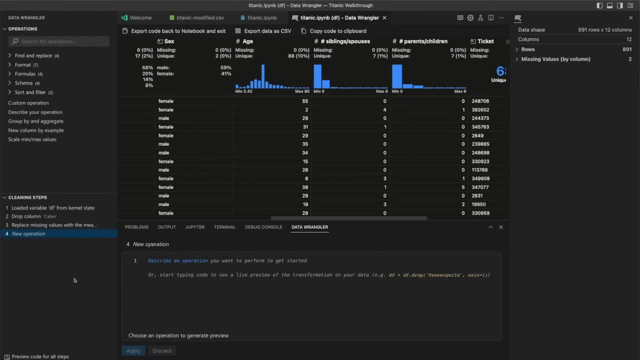 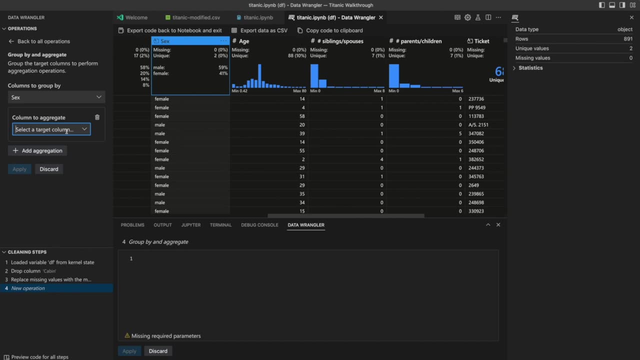 can be referred to at any point by just a simple click. Now that we've removed the missing values, we'll want to see if the age old titanic motto of women and children first told true. We can use the group by operation on the sex column and aggregate on the survive column to get an answer With just a. 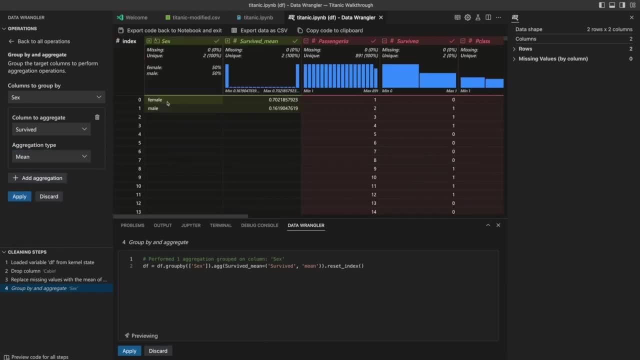 few clicks we can see that at least the first part of the motto is true, with female surviving at a much higher percentage, at 70% compared to just 16% for males. In addition to this, we'll want to see if the second part of the 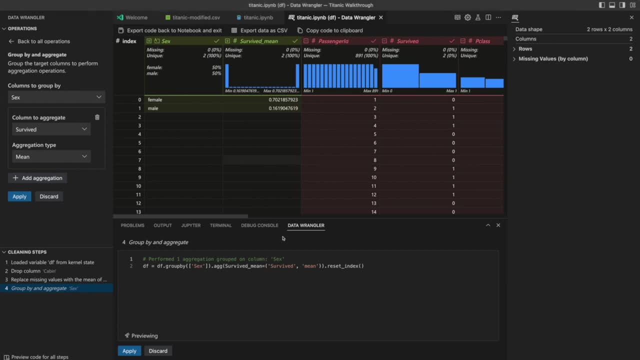 statement is true. by seeing if age affects survivability Again, I can quickly modify the code to create five different age intervals and perform the group by based on that interval. Again, we can see that children had the highest chance of survival at 55%. 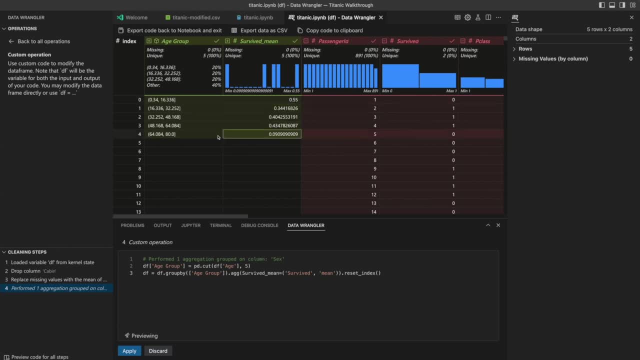 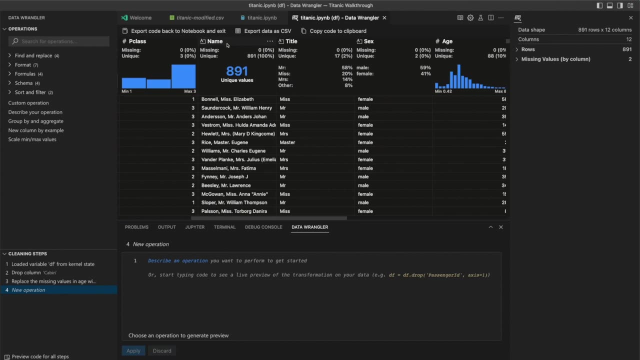 and seniors had the least, at just 9%. This is a good smoke test to determine that the columns of sex and age may be of interest and importance to this dataset. Another thing we can do with the titanic dataset is to featurize the passenger names by extracting out their first name. 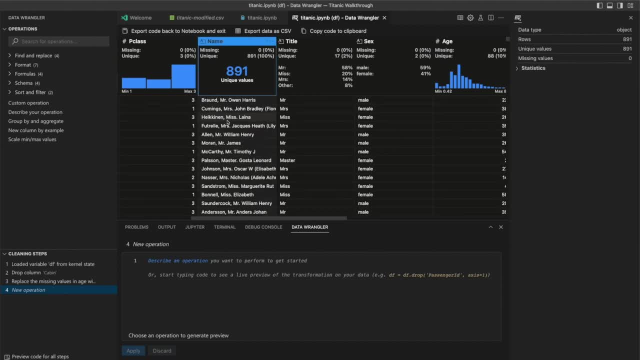 We can see that the named data is unclean. some passengers have various titles, like Mr, Mrs and Master, and some folks have middle names. some folks have nicknames and some folks don't, so this is not a simple extraction task. Fortunately, we can leverage the built-in data. 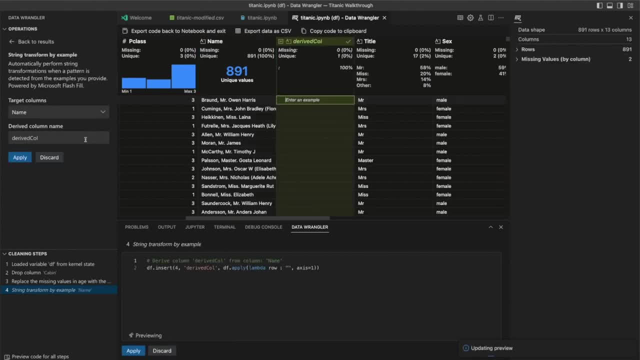 wrangler operation called StringTransformByExample to extract out the first name. How it works is you give it an input column to analyze. so in this case the name column In the new empty column can provide examples to data wrangler about what we want to extract out from the input column. 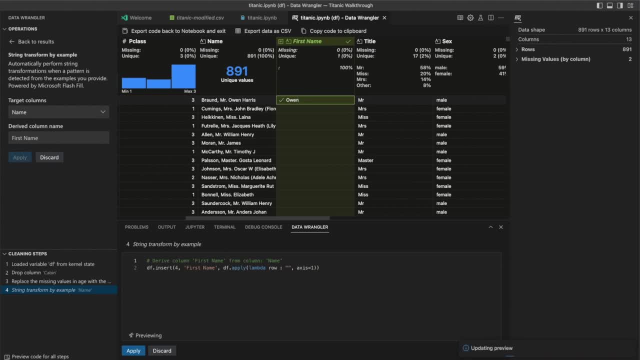 So in this case, for the first row, we'll say we want to take out the word owen. Data wrangler will then try to interpolate the rest of the values in the column based on the example you gave, And you can see here it does a pretty good job of extracting out the first. 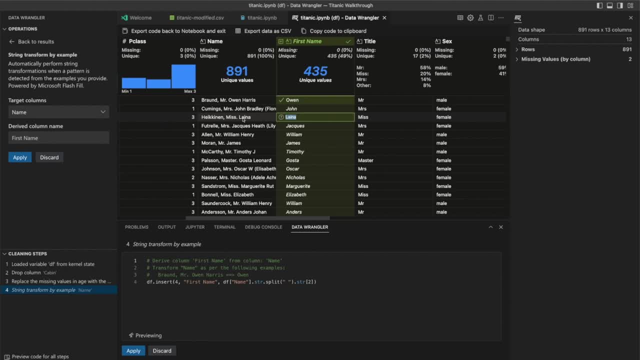 name, even though the passengers have various names and various titles. If one example is not enough, you can actually modify or give additional examples to data wrangler. Finally, you can again also get to see the exact piece of python code that was used to perform this extraction. 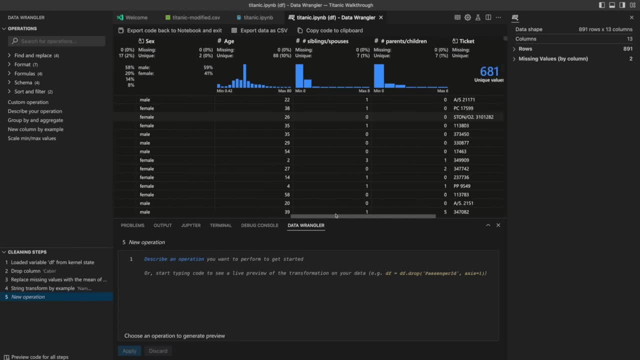 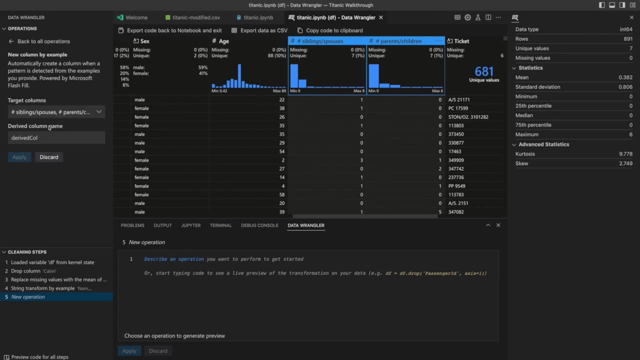 One additional thing we'll notice in this data set is that it contains both the number of siblings and spouses, as well as parents and children, as separate columns. We can reduce this down to just one column of the number of relatives to reduce the dimensionality of this data set. To do so, we 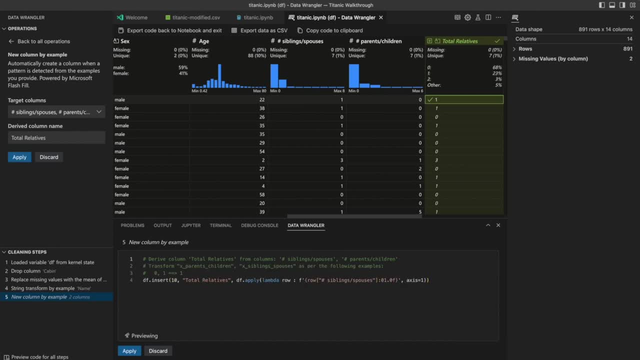 can leverage the new column by example operation. We give the first row an example of one and if we look at a few examples, we'll notice that for the first row we'll see that the first row is the first row and the second row is the second row, And we can also analyse the second row and it. 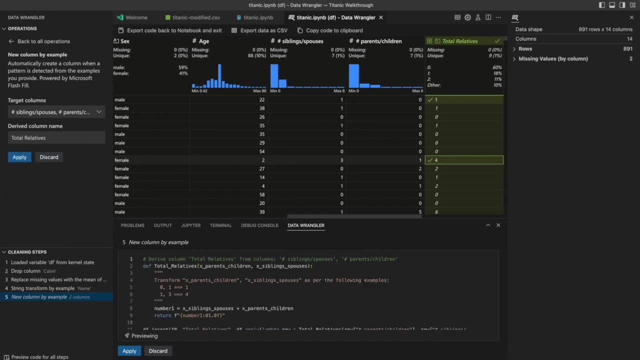 didn't add the three and one correctly, So I can update the example to say four. Now, once the code is regenerated, we can actually see that it adds both columns correctly together. There are many other things I can do with this Titanic data set, but again, once i'm happy with the progress, I can 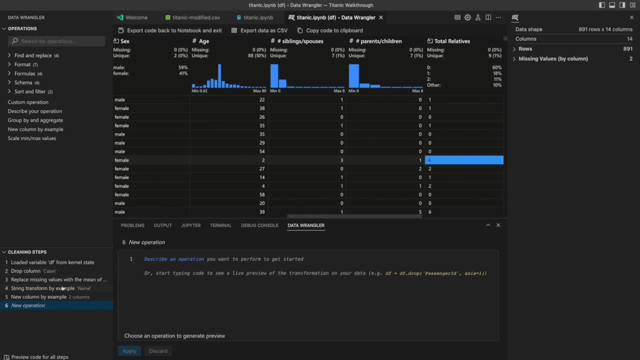 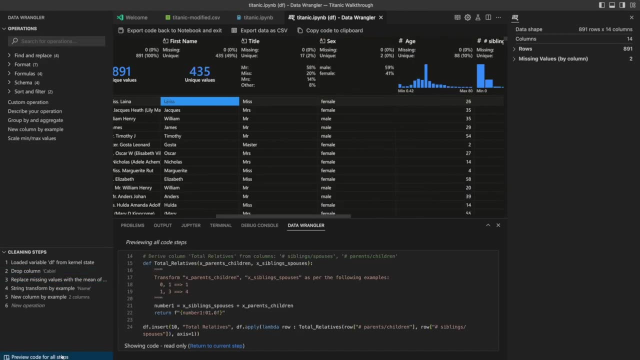 actually review everything that was done from the cleaning steps panel as a sanity check, to both remind myself of how I got here as well as if everything I've done makes sense. I can also take it a step further by clicking preview code for all steps to see the exact python code that was. 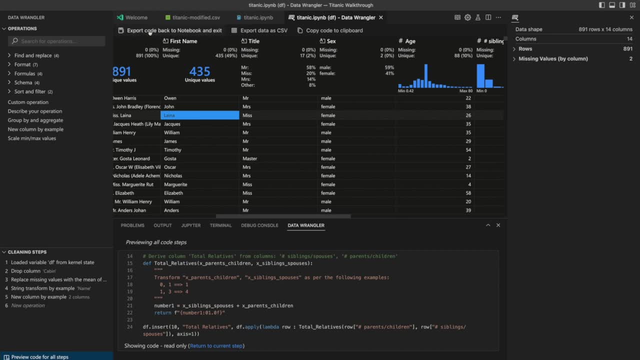 generated to get me here. Once everything looks good to me, I have several options to choose from of how I actually want to export this clean data set. From the top export menu, I can either export code back to my notebook, export the code to a. 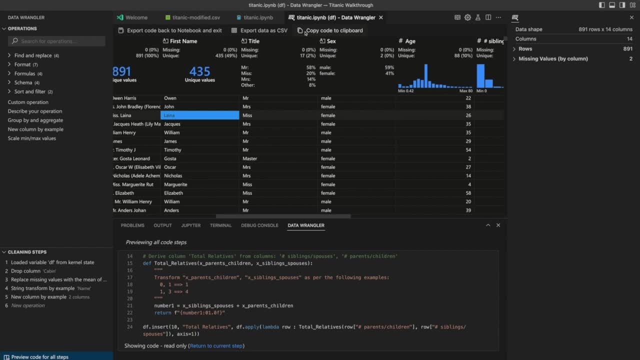 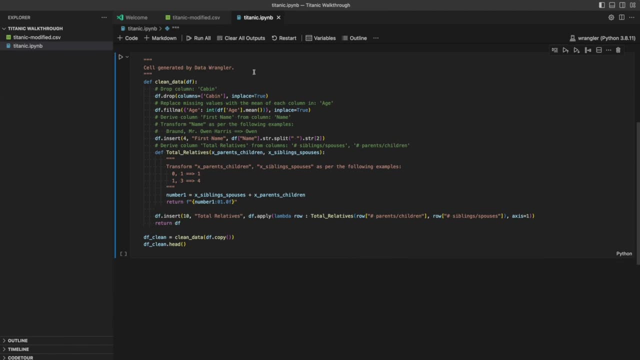 new CSV file or even copy the code to clipboard to be pasted into any Python script. In this case I'll export it back to my notebook so I can pass it to my machine learning model. Once the code is back in my notebook, I can execute this. 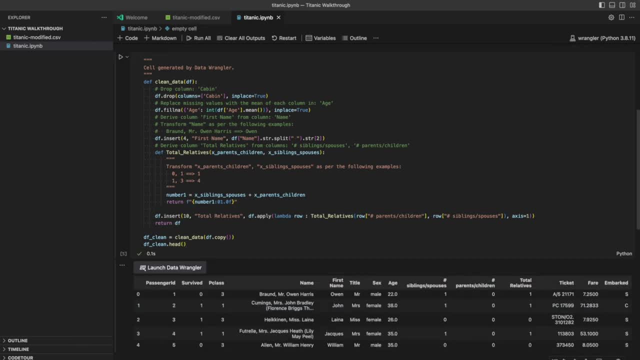 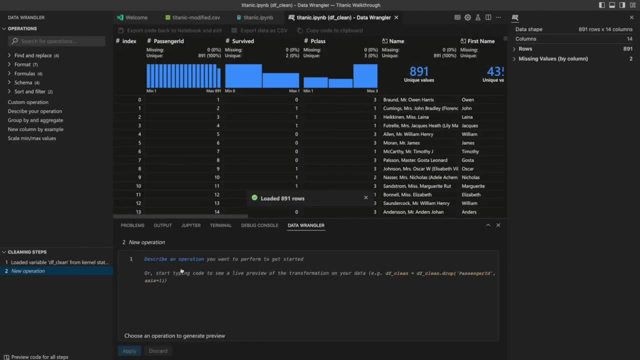 code and anytime I have a data frame now within my notebook and want to do some additional analysis in the sandbox environment of DataWrangler, I can just pop back in anytime with a single click of launch DataWrangler. In summary, what we did today was to explore and clean up the Titanic data set with DataWrangler. 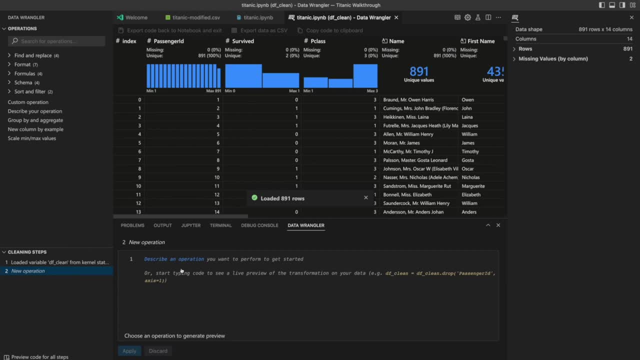 We started by launching DataWrangler from my Jupyter notebook. performed some exploratory data analysis on the data set using the quick insights and summary statistics. performed some data cleaning with the built-in operations such as replacing values, as well as use the by example operations to have DataWrangler.